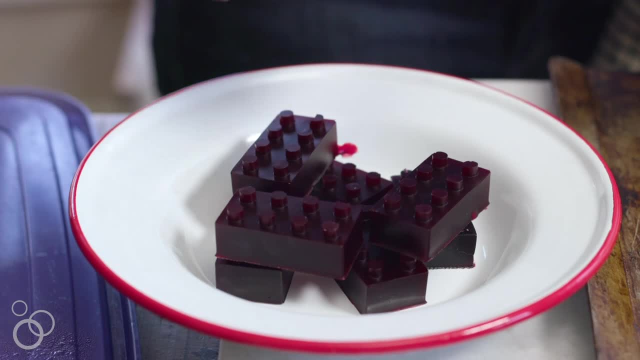 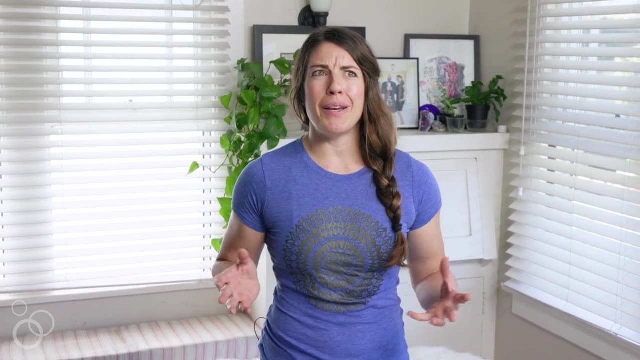 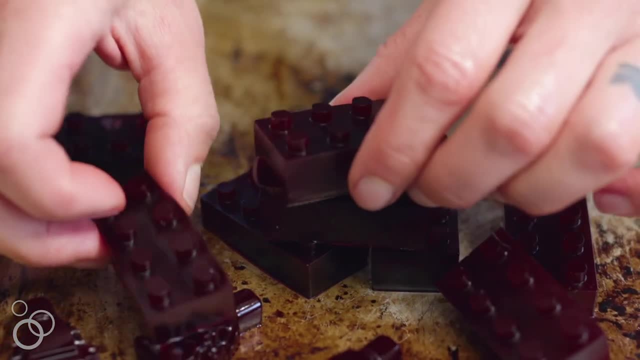 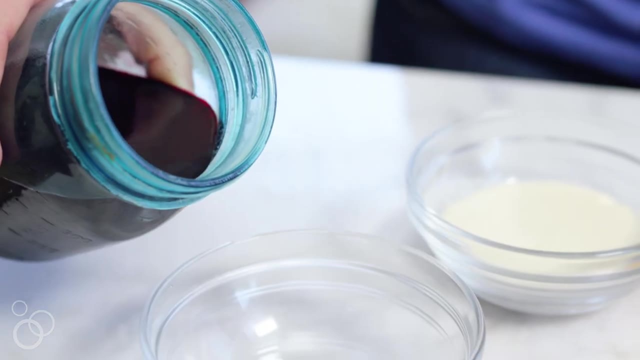 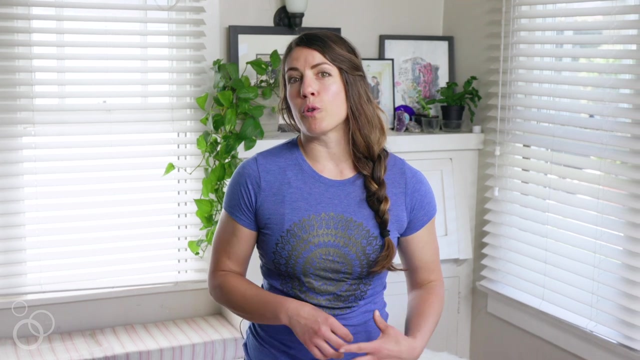 Use whatever shapes that you really like To make this recipe. all we're going to do is get our fruit juice, and you can use any kind of juice you'd like. I really like beet juice. Why? Because it's a little subversive. You're going to be sneaking in some really healthy stuff, Beet juice. 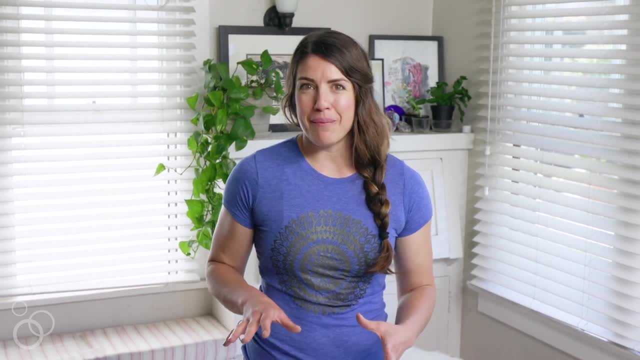 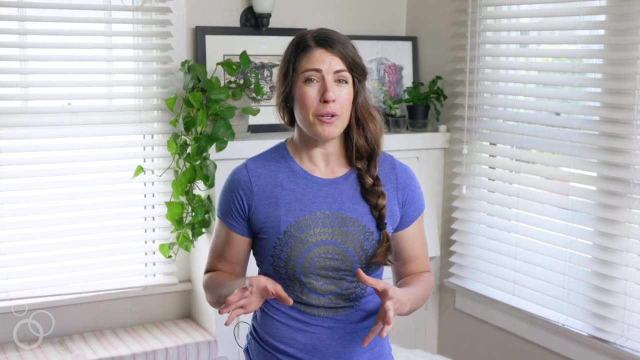 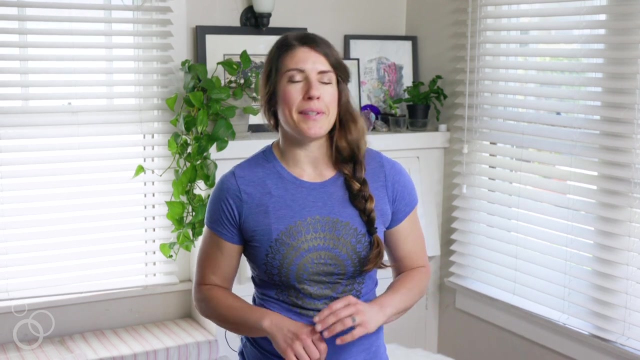 is great for your liver and it's got lots of amazing vitamins and minerals. So I love beet juice and it has a vibrant red color that is just so enticing, especially for little kids. They love the red color of that. but it doesn't have any fake food dyes- red number 40, none of that stuff You can also use. 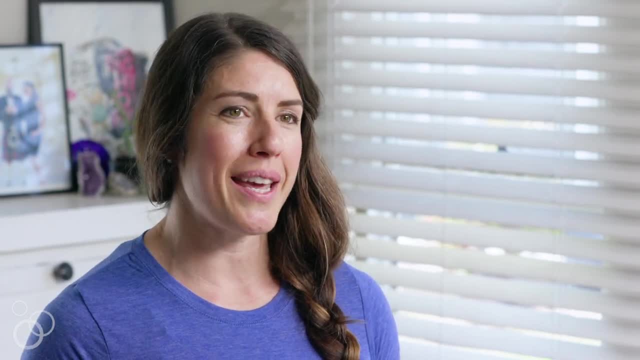 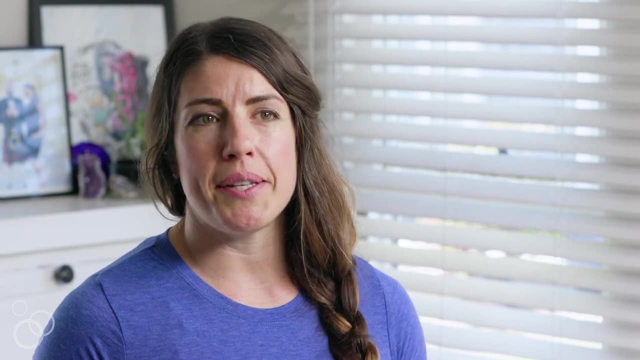 grape juice. That's another one that's really great for this recipe. I would just steer away from things like pineapple or mango or anything that's kind of a tropical fruit. The reason is it will actually cause the gelatin to not harden up, So try to stay away from those juices. but you've got. 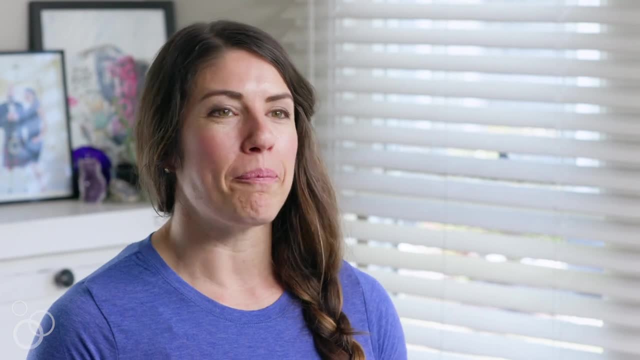 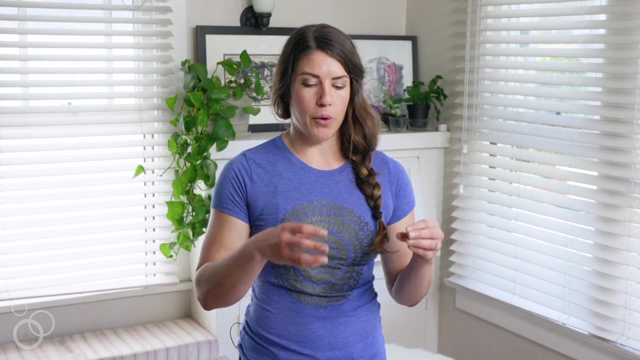 lots. you know the world is your oyster here. Pick what you like and run with it. All we're going to do first is bloom the fruit. This is a really important step. If you don't bloom your gelatin, it's going to get clumpy and hard, and nobody likes that. So to bloom the gelatin, you're going. 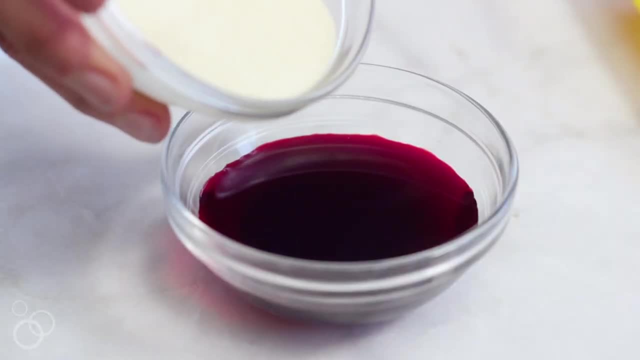 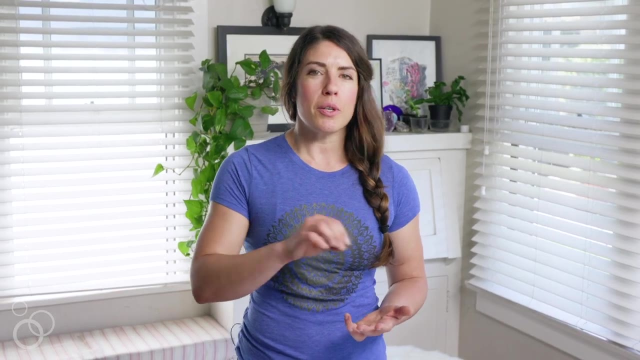 to take a small amount of juice, either room temperature or refrigerated, and you're going to sprinkle the gelatin on top. I like to kind of stir it in with a chopstick just to make sure that all the little gelatin particles get softened. That's what blooming means. It means that when we add, 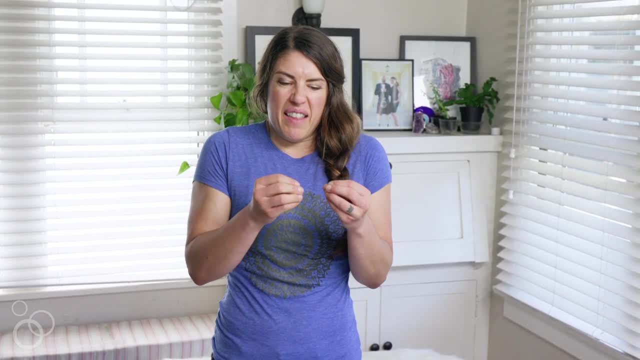 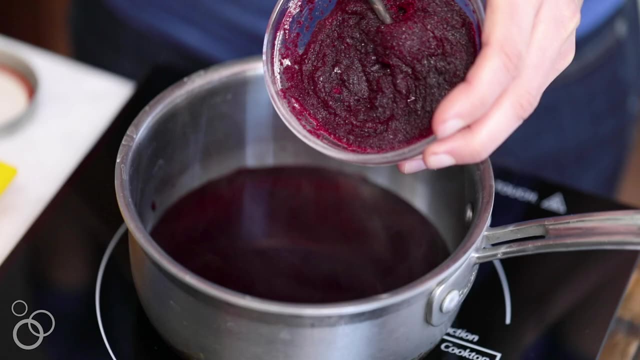 our hot liquid. it's not going to seize up and make these hard little, clumpy bits that nobody really likes. Once the gelatin is bloomed, we're going to add that into the rest of the juice which we heat.